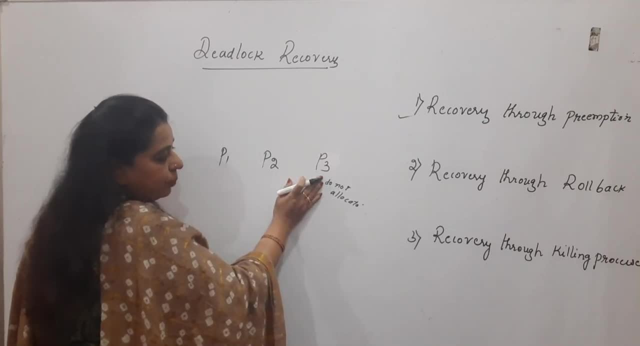 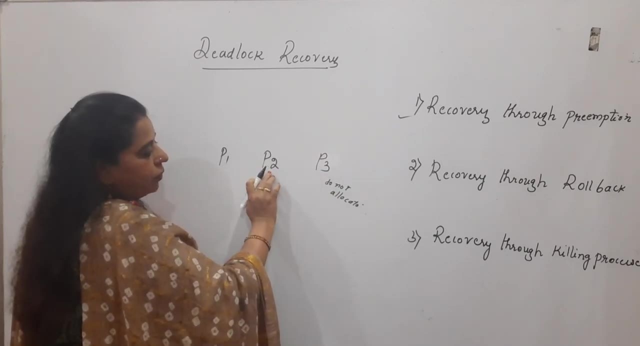 In this situation, suppose after deallocating the resources from P3. still, if you feel that there is a deadlock occurring, then carry out the same procedure for P2.. Deallocate the resources from P2 and see that whether the system will result in deadlock free. Always to the previous point, you 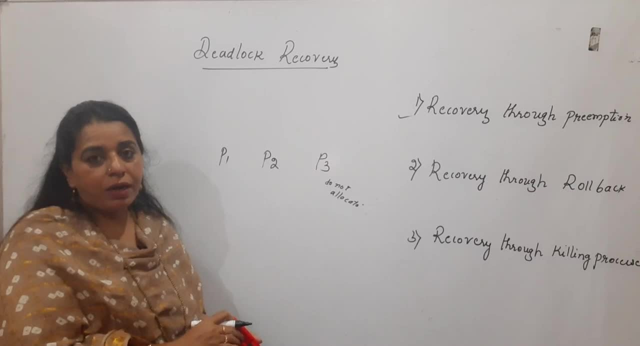 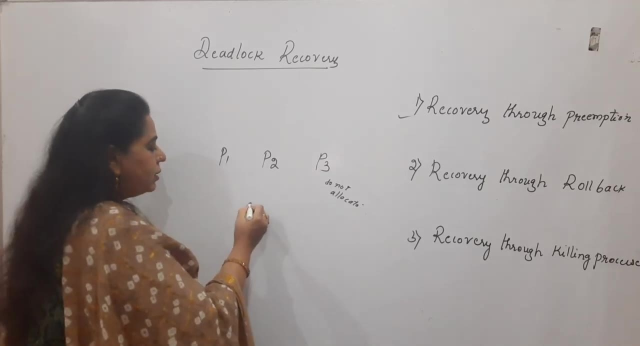 have to move so that and try to see that there should not be any deadlock in the system. Moreover, at this point you have to be very carefully in selecting the processes. Also, see that the processes do not get starved. Starvation should not happen, because in this method you are going. 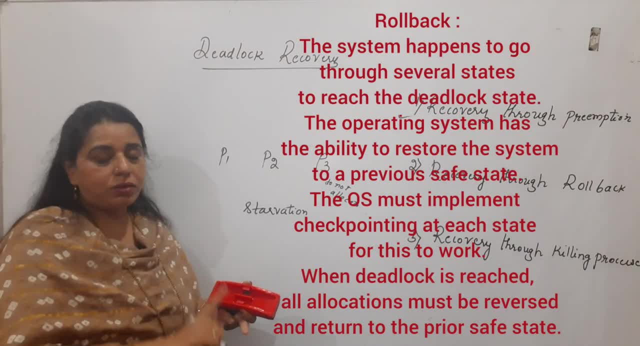 to deallocate the process from the deallocate the processes. In this method, you are deallocating or you are releasing, or you are making the resources to be released from the processes. So you are selecting one particular process. Meanwhile, while selecting that process, you have to also see that how much percentage of job that process has. 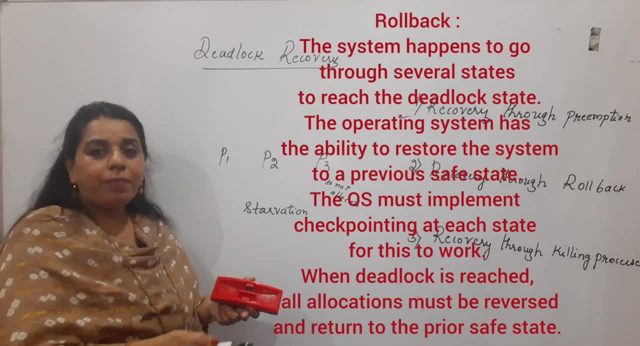 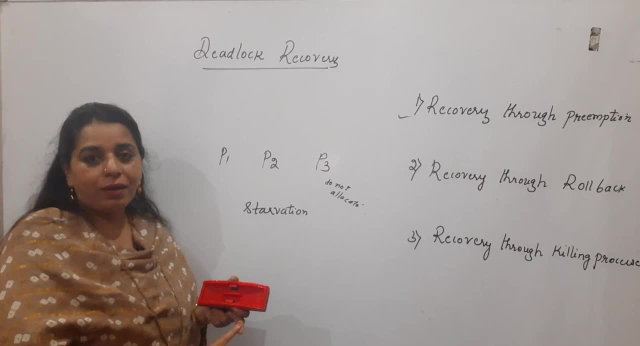 completed. So releasing the resources when a process is almost about to complete its job is a very costly affair. in the system You are not supposed to do that A process which is initially in the beginning of its execution. you can choose that process to be released from the deallocate. 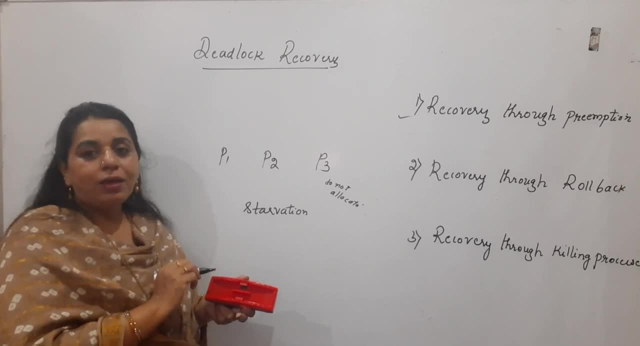 It will be a process to what? To make the process, release the resources and also, when you are carrying out this method, see that one particular process is not always chosen to make the system become from deadlock free. Otherwise, that process will never be completing its job, so it will always. 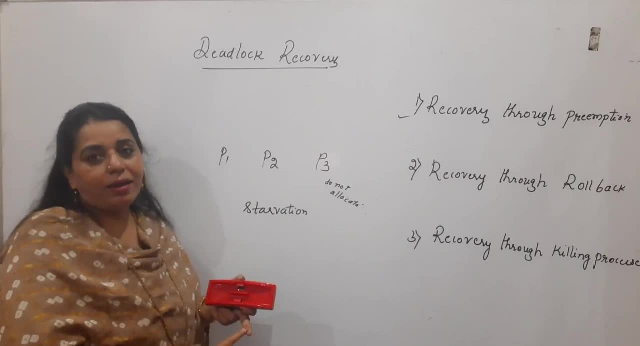 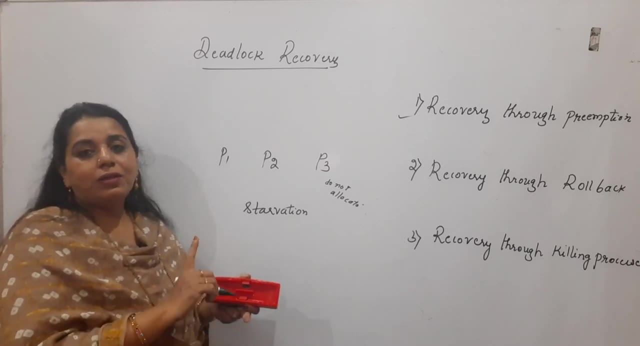 be what, waiting, and it we say that there is a starvation occurring in the system, that also you should see that you are not going to penalize any one particular process all the time in the system through recovery. and then you have recovery through killing process: killing- 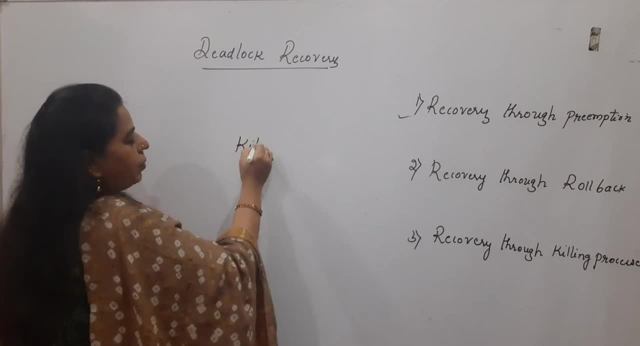 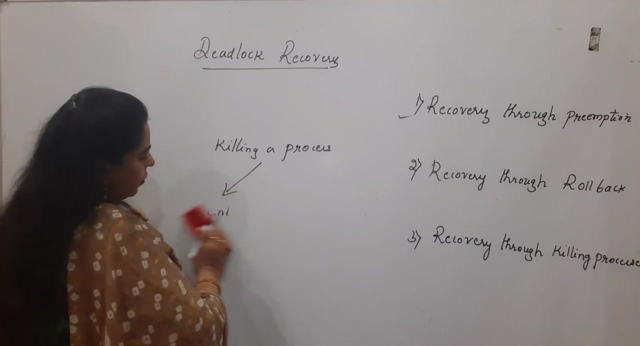 process is also what. once again, keep in mind that whenever you kill a process, see that how much percentage of job a process has completed. normally there are two ways here. first, you can kill the entire, all the processes, all the processes. if you try to kill, what does it mean? all the processes in the system? 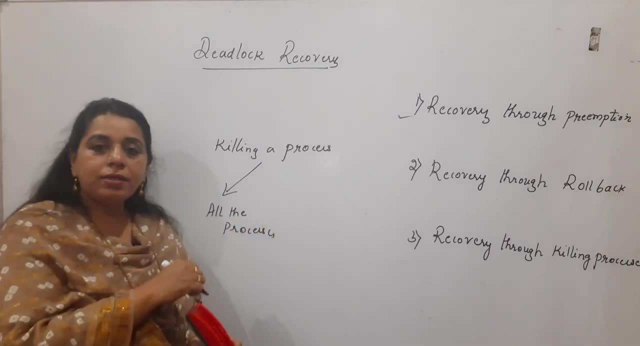 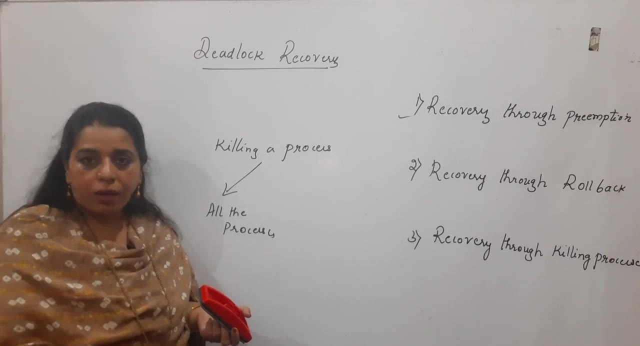 are killed once you kill all the processes in the system. the reason for killing all the processes- the processes I have resulted in a deadlock in the system. okay, because they are not able to complete the job. better to kill all the process and start reassigning the resources again, so that you will see. 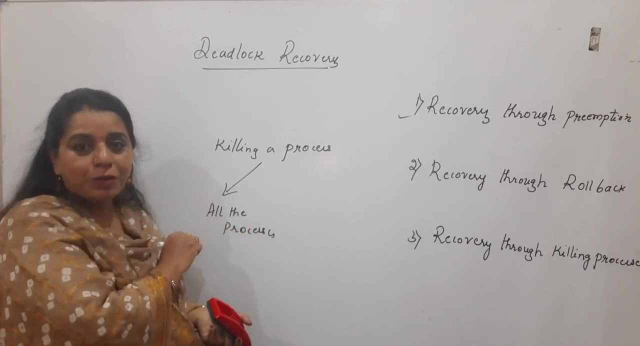 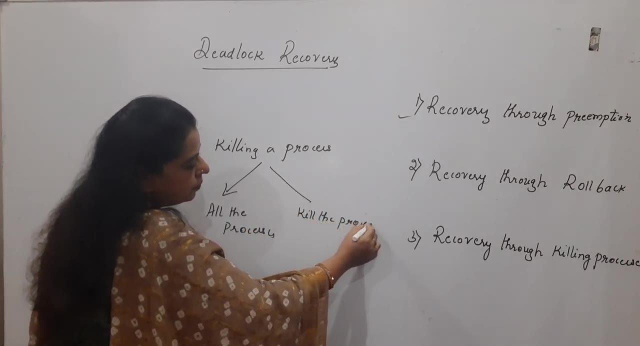 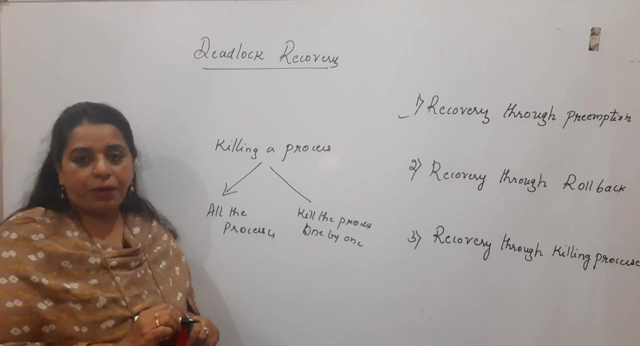 that there should not be any deadlock in the system. so we say in that manner also, we can recover. otherwise you have, kill the process one by one. one by one is terminate one by one process first, okay, and then see whether the system becomes deadlock free. so why? 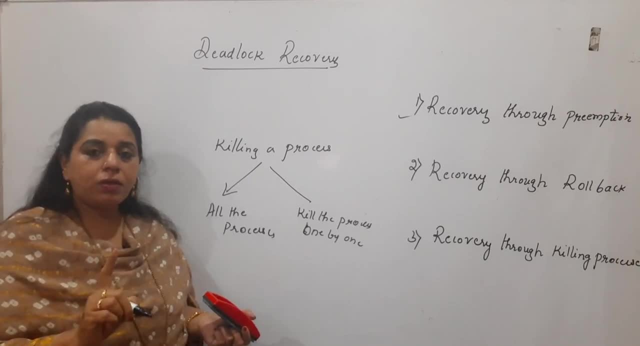 to kill all the processes unnecessarily just by killing one process. also, if you are able to make the system deadlock free, then the other processes cannot complete their execution. so but to I add, you have to identify that process in a very intelligent manner, see normally. I'll tell you one simple example. if 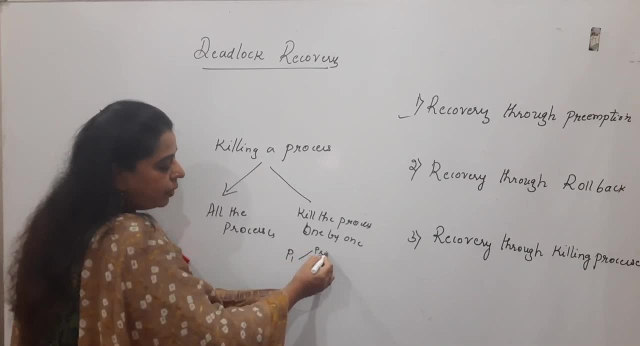 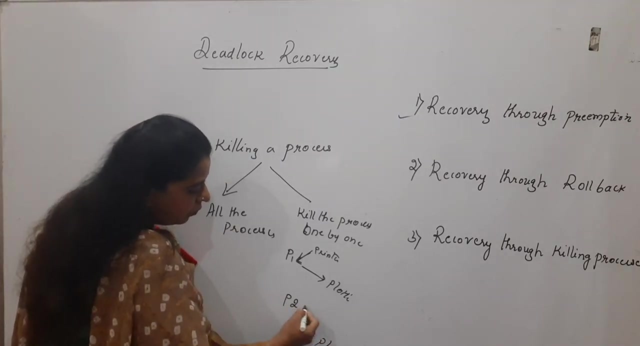 there is one process, p1. p1 is requesting for printer. okay, actually printer is assigned to process p1 and it is requesting for plotter. there is another process, called p2. p two is assigned with plotter. okay, but it is requesting for printer. there is one more. 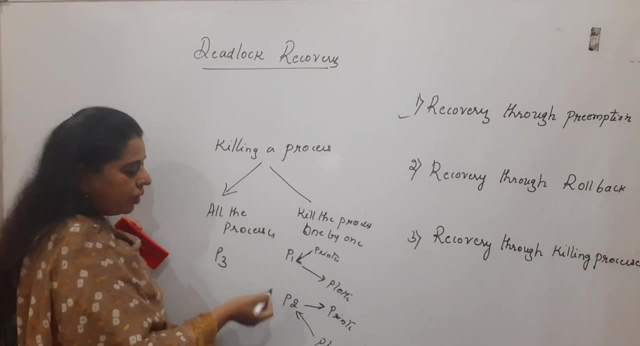 process p3. ok, the system is having two instances, more than one instance, of the printer. p three is a assigned with one instance of the printer. p 3 is also as with one instance of the plotter. okay, so this p3, which is 1 of printer and 1 is 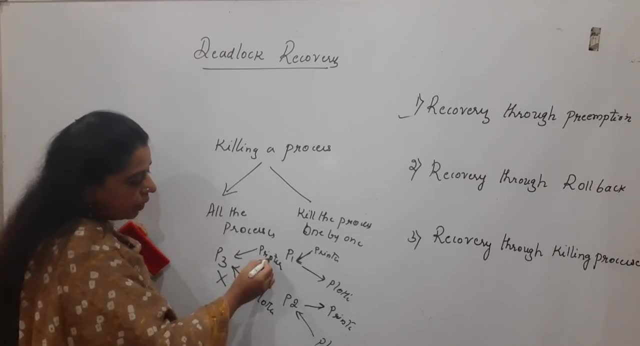 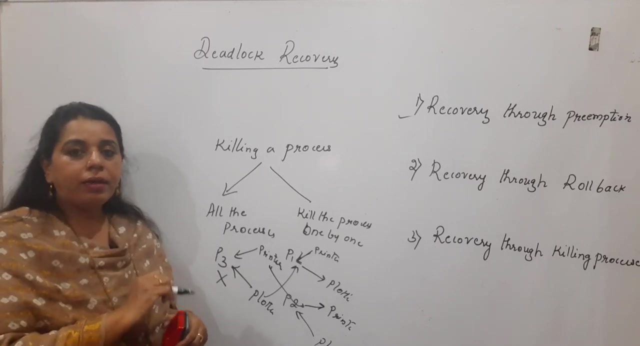 of plotter. if this process is killed, then this printer becomes available. this plotter becomes available so that this plotter can be what assigned it to this p1 printer can be assigned it to this p2, and p1 and p2 can complete their job this way in a very intelligent manner. the process to be 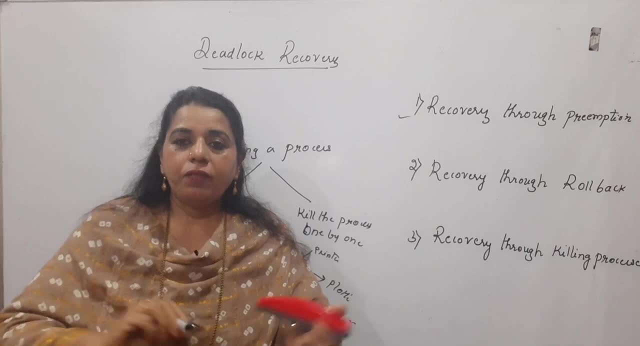 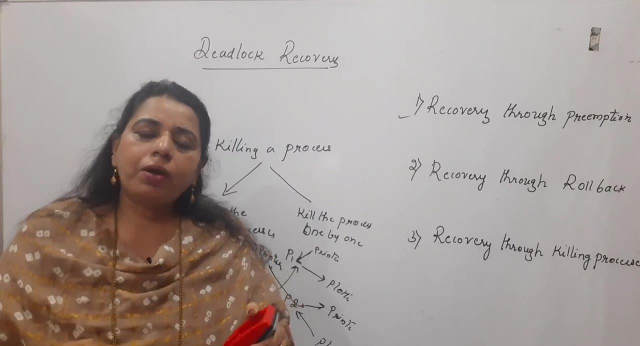 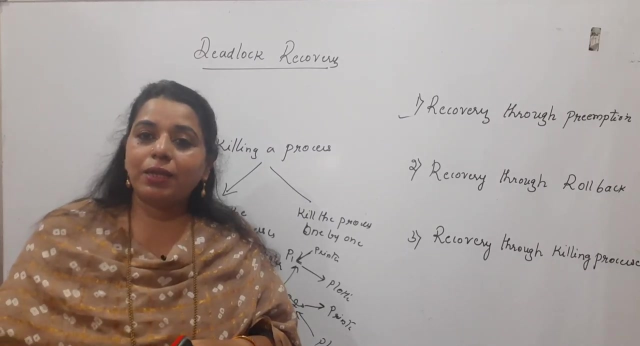 killed has to be selected. normally this is what it will happen if a system is having, suppose, some p1, p2, p3, some 10 processes. you just assume there is one process which is holding maximum instances of all kinds of resources, so that particular process is itself making all the other processes. 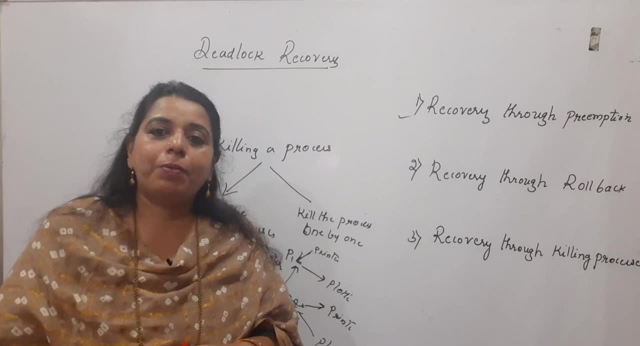 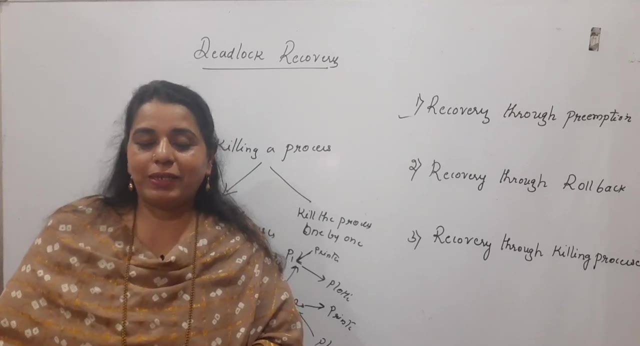 to wait, so better to kill that process. once you kill that process, all the resources become available, and all those resources will be what allocated to the different processes which are requesting, and the rest of the processes can complete their job. so this is how you have to carry out what